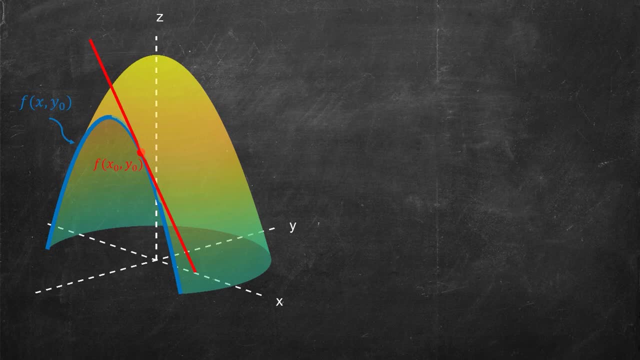 can answer back in first-year calculus. The only difference is that we have this y naught being floated around. This is the idea of a partial derivative. So the formula for a partial derivative is a bit of fancy notation. It's a sort of weird script thing that looks a little bit like d and I. 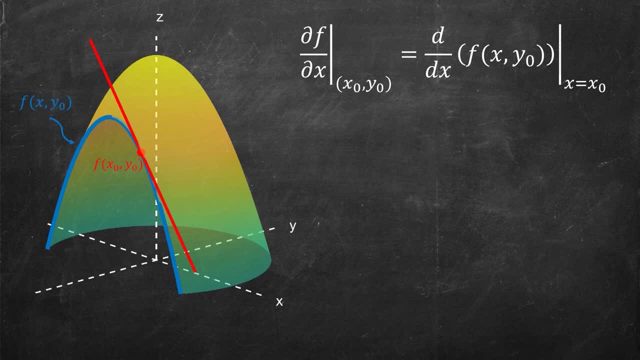 pronounce it: the partial of f with respect to x. That's what that del f over del x is Is another way of saying it, Typically: the partial of f over the partial of x. I'm evaluating this at a particular point. x naught, y naught The answer to what this new thing is: these partial. 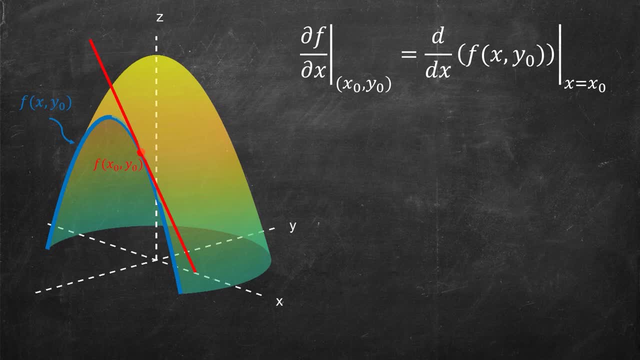 derivatives is: is it simply the old derivative of a one-dimensional function, that one-dimensional function f of x comma y naught? Which is to say that after I plug in the y naught that function only depends on x. And so I can take the derivative using the old d dx notation we use. 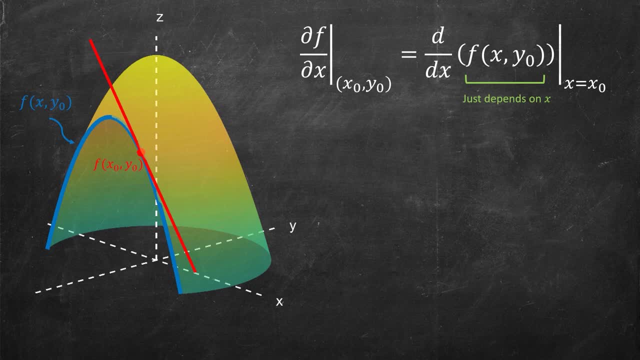 in one dimension, it perfectly applies. Finally, they use the long vertical bar to evaluate it at x equal to x- naught. So the idea is that I have defined the partial derivative of a multi-variable thing to simply be the original single variable derivative when I plug in the value y- naught. 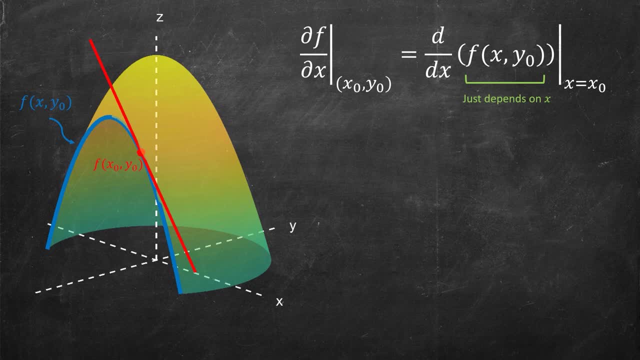 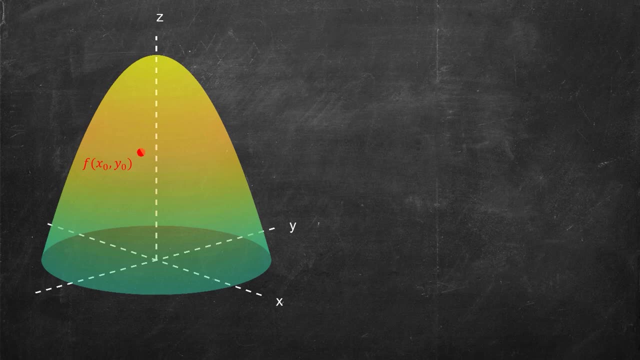 This is the partial derivative with respect to x. We can also investigate the partial derivative with respect to y, So let's begin in the same place. I have about that graph of my function. I have a point specified, But this time I want to restrict myself where the 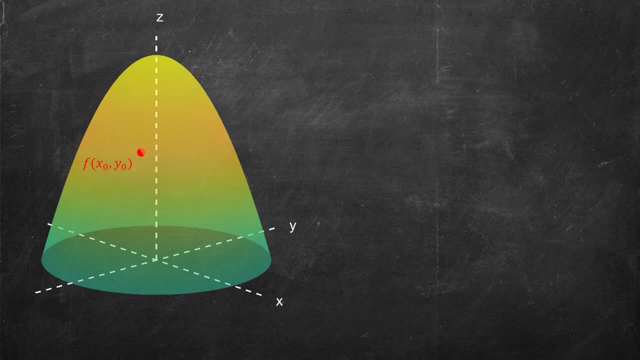 x naught value is fixed and the y value is changing. That is, I'm on a plane here with a fixed x naught and then all the values of y that are allowed. When I can take the intersection of that plane with the graph of my function, I cut away. what I get is nothing but the equation. 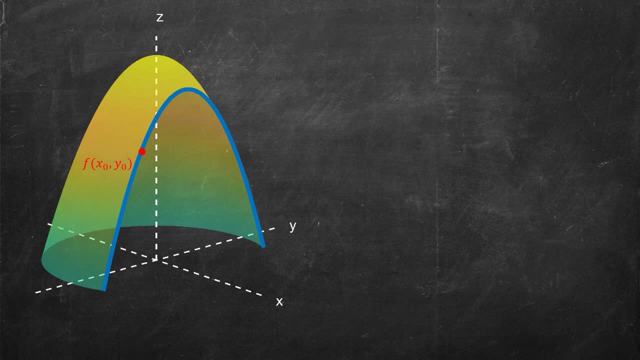 of a parabola again. It again looks like something that is a one-dimensional function. Indeed, this blue portion can be thought of as the function where I plug in the value of x naught and I allow y to be arbitrary, So it has one now: input that varies. It only has the input y varying. 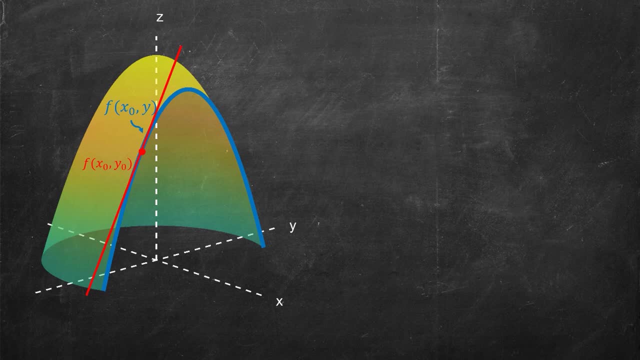 So from this I can also ask: what is the slope of the tangent line to this f of x naught comma y? And the slope of that tangent line is a question that we can answer in first-year calculus. Hence I'm going to define my partial derivative. 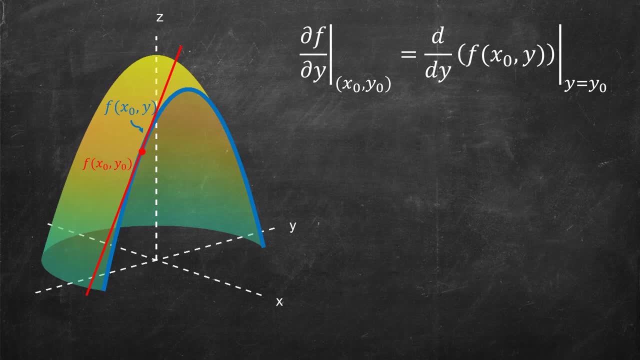 I will say that the partial derivative of f with respect to y, evaluated at the point x naught y naught- that's what the long vertical bar means- is nothing but the single variable derivative d, dy of this function that only depends now on y. This function f of x naught on y. 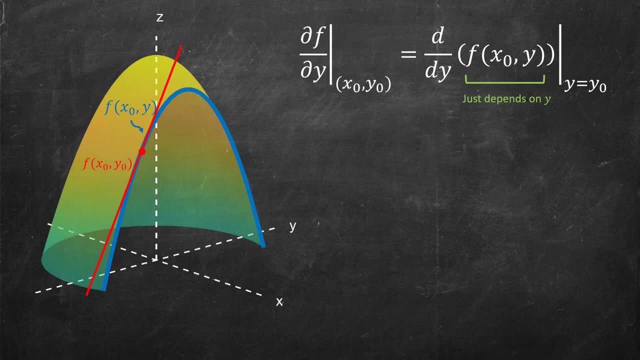 Then, finally, when you plug in the value of y equal to y, naught, you've now figured out what is the slope of the tangent line to this f of x. So that's what I said in the first-year calculus. So the slope of the tangent line is the slope of the tangent line within the y direction. at this point, x naught, y naught. 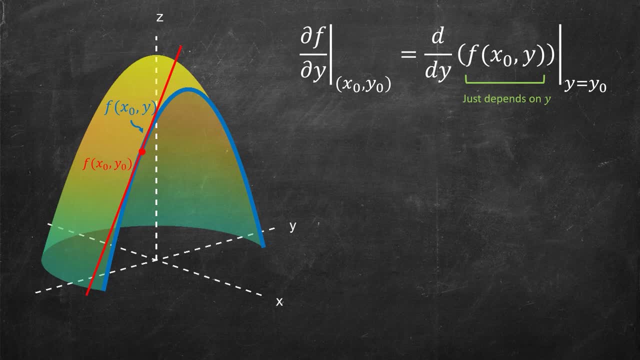 So the way I interpret this geometrically is that the partial derivative of y is what happens if I walk along my surface, the graph of my big function, but with the x value fixed. In other words, it's the slope if I walked only in the direction parallel to y. 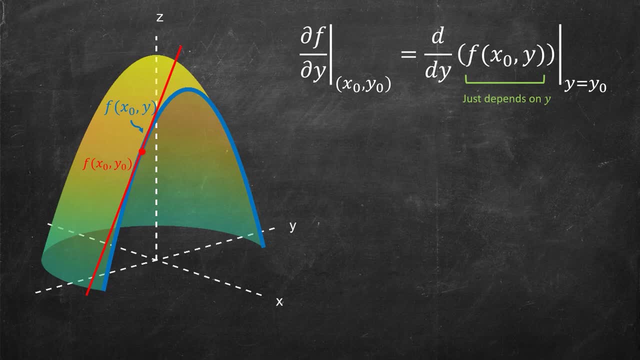 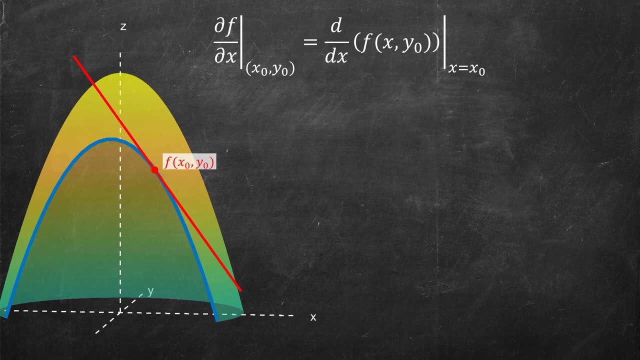 only in the x-directional on my surface. how steep is it as I walk in that direction? Let me rotate my view a little bit, and I'm talking about the partial derivative with respect to x. I want to try to dig a little bit deeper into this process. Recall that we had the one 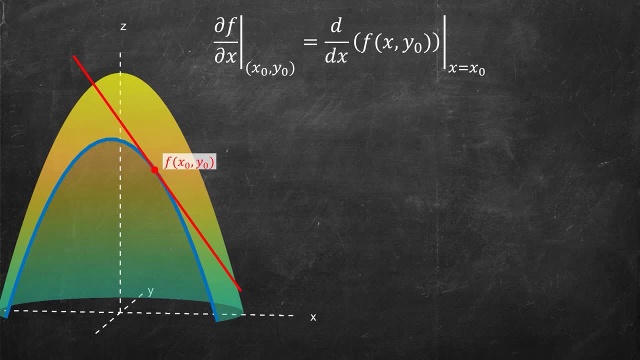 point put on the graph f of x naught, y naught. but how was derivatives defined back in first year calculus? Well, the idea was that you would consider the slope of the tangent line to be a limit of the slopes of secant lines. The way we did this is that we would put a second point on 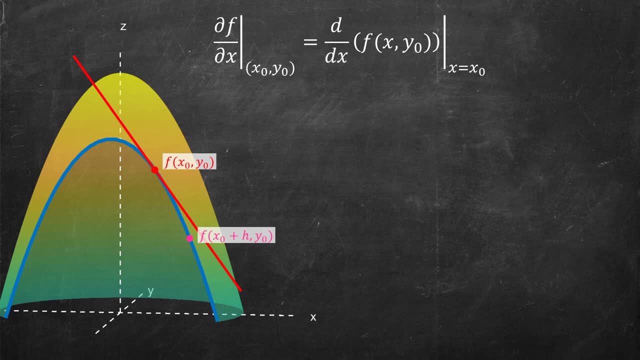 some other point that was also on the graph and I would put on the point. it will be pink labeled: f of x naught plus h minus y naught, That is, it has the same y naught value. This just wasn't relevant in first year calculus, but nevertheless, what's. 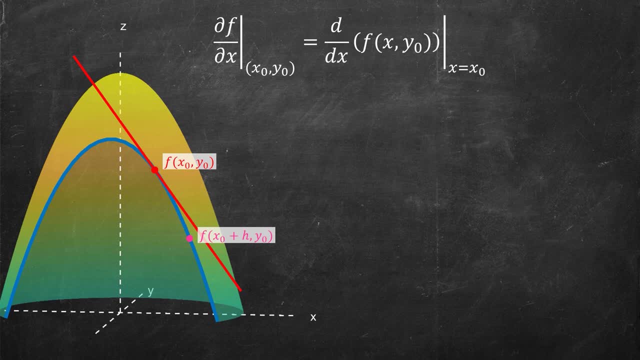 changing is the x value is going from x naught to x naught plus h. Then when you have points on a curve, you can define the secant line that goes between those two points. Then I can ask the question: what is the slope of that secant line, What is the rise over the run? And, in particular, 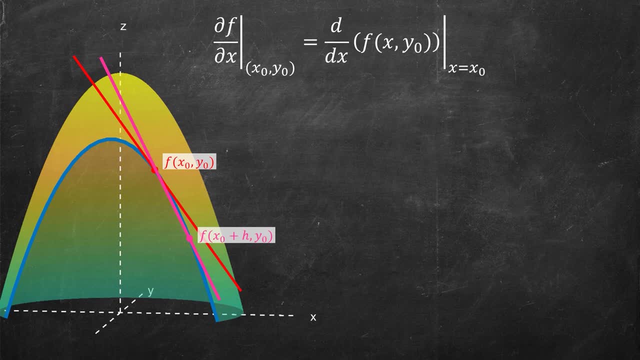 as that h value gets closer and closer and closer to zero- in other words, the two points get closer together- then the slope of the secant line is going to approximate the slope of the tangent line. So if I want to do this, I'm going to have to do this. I'm going to have to do this, I'm going to. 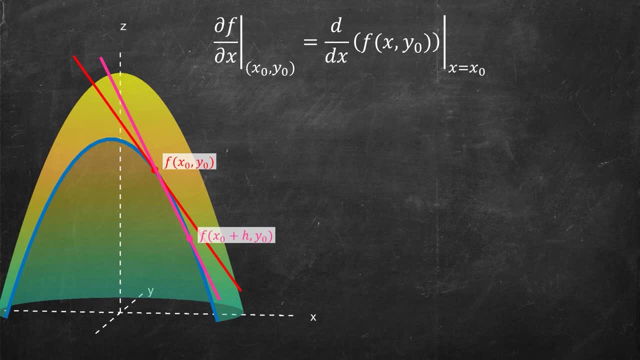 do this. So what we defined the derivative back in first year calculus to be, and to which we can extend it for these partial derivatives, this is nothing but the limit, as h goes to zero, of the rise over run for this secant line, the slope of the secant line And the change in the y values. 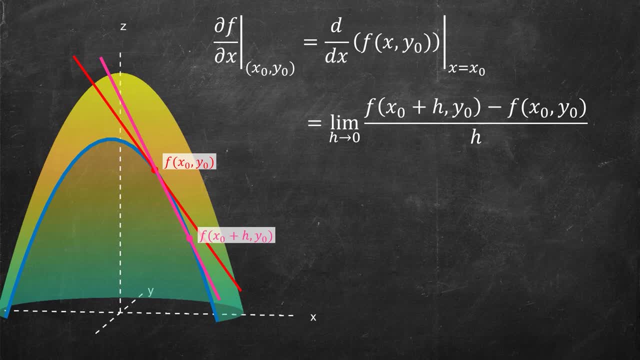 the rise is f of x naught plus h, minus y naught, minus f of x naught y naught. That's the change in the output values and the f values And then the change in the input values. you went from x naught to x naught plus h, so you divide it out by h. 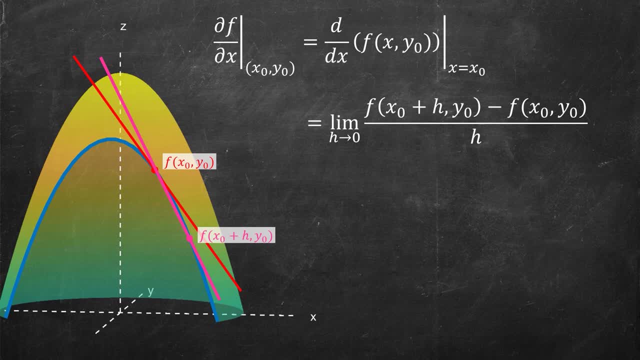 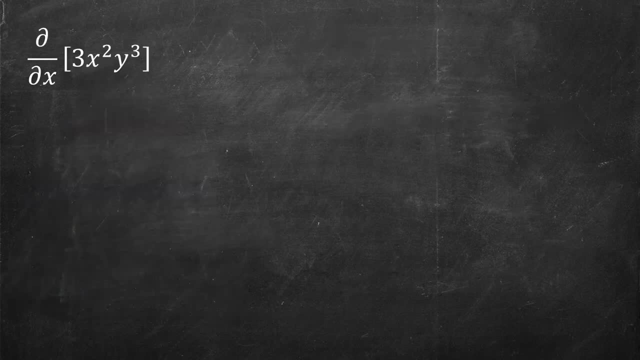 So this is our formal definition of the partial derivative of f with respect to x in terms of limits. Let's investigate how to compute this thing. When I think about just the partial derivative with respect to x of, say, the function 3x squared y cubed, I haven't evaluated any. 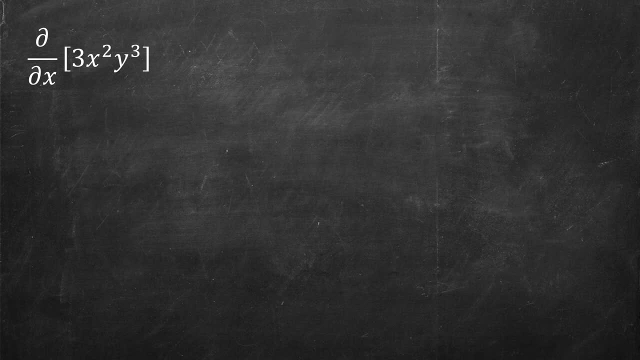 specific points. I want to do it in general. The way I'm thinking about this is that, because I am taking a partial derivative with respect to x, I'm taking a partial derivative with respect to x. y is fixed, y is constant, It does not change as I'm changing the value of x And because it's 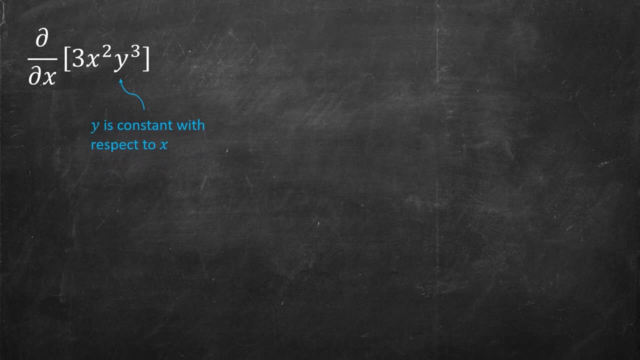 constant with respect to x, that is when I take its derivative. I can treat it the same way as if it was, say, 7 cubed here, in which case 3x squared times 7 is easy. You just do the power. 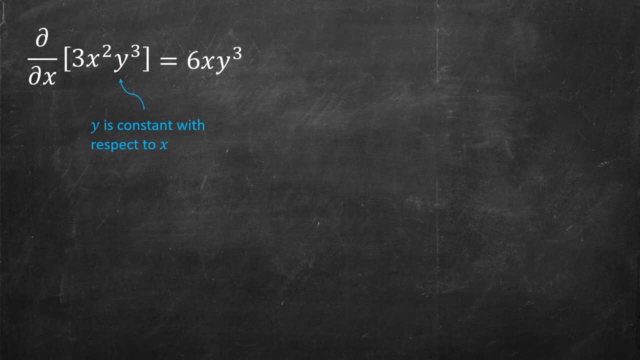 rule and you say it was 6x times. whatever the constant was, in this case y cubed. So computing partial derivatives is just a question of everywhere there's a y, you just imagine it's a constant. You take the derivative with respect to x as you would have. 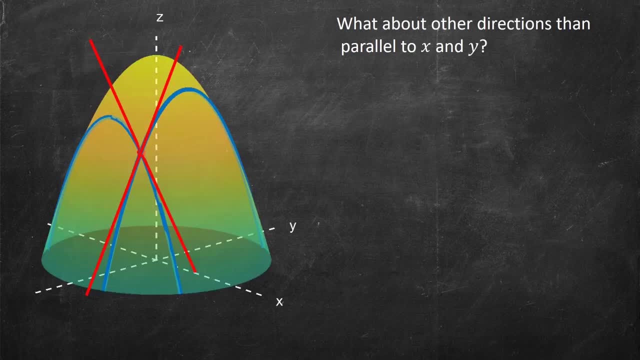 done before. Finally, I've given the image where I've put both of our two answers. At my particular point, I've shown the curve that happens when you move only along x and the curve that happens when you only move along y. There's two different tangent lines to those two different curves.